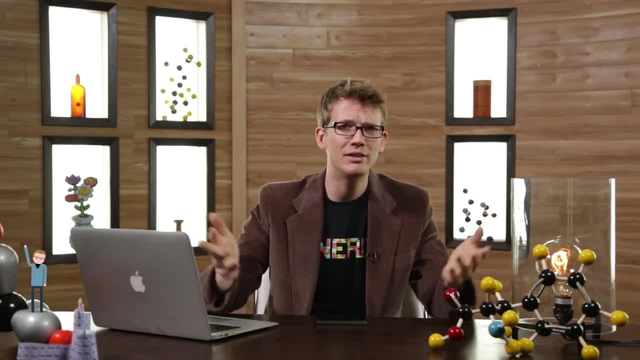 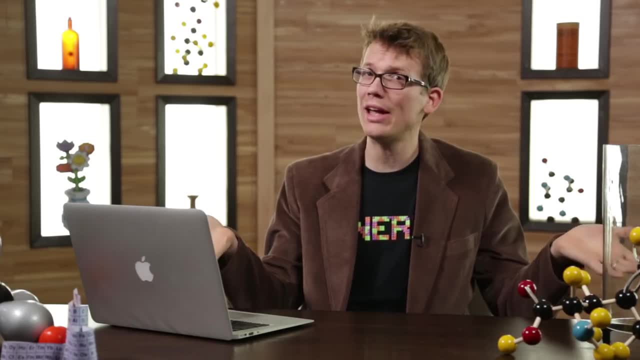 You got a pretty good idea what chemistry is right. It's atoms and molecules doing stuff and making cars and food and life and everything, And of course it's the study of those things. But like, how did we get here? 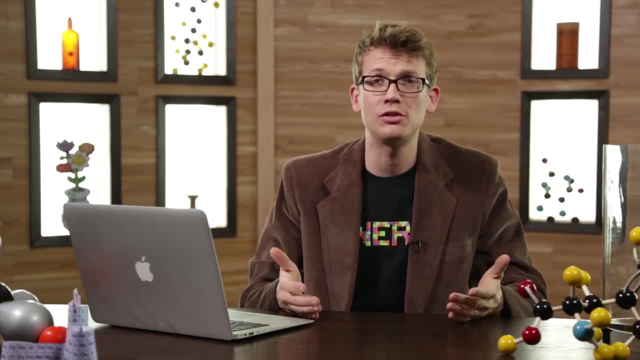 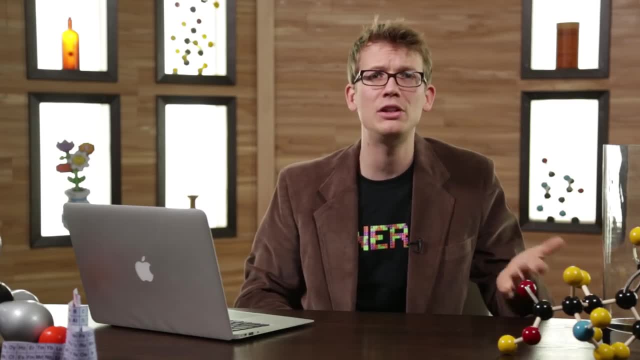 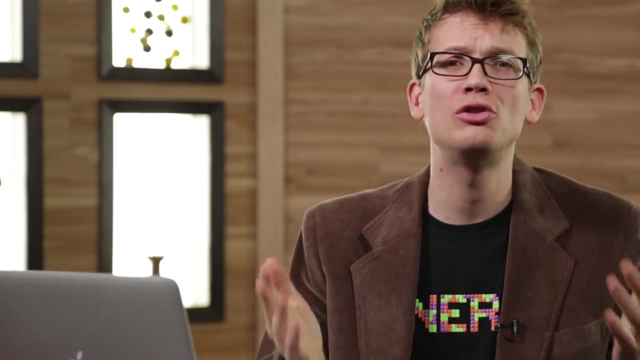 There's certainly no everyday evidence for much of what we have discovered through the science of chemistry, Discoveries that were not derived or made up, but just laws of the universe that exist simply because the universe is the way the universe is. So in today's episode of Crash Course Chemistry, we're going to be taking a bit of a historical perspective. 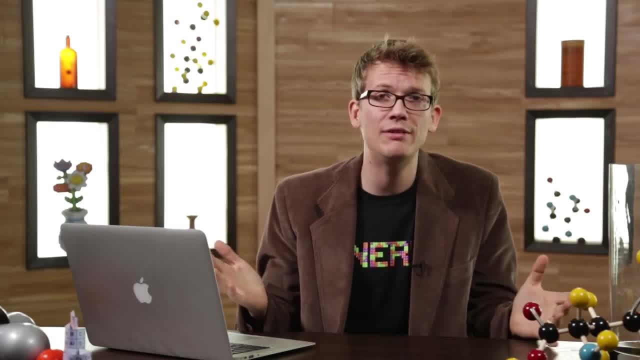 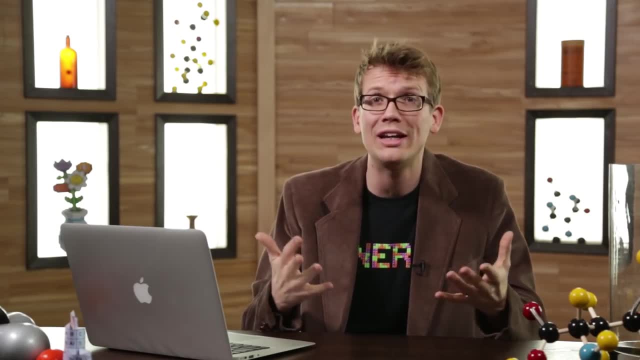 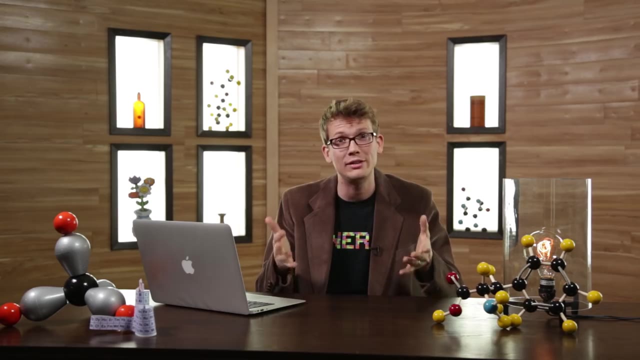 on the creation of the science of chemistry, A science that didn't really even exist until a super smart, super wealthy French guy put the puzzle pieces together into a coherent theory for, quite literally, how everything works. And if you've ever found yourself sitting at your desk reading the same line in your chemistry book the 22nd time, 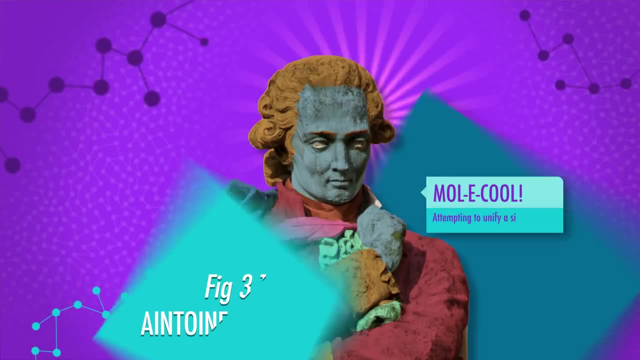 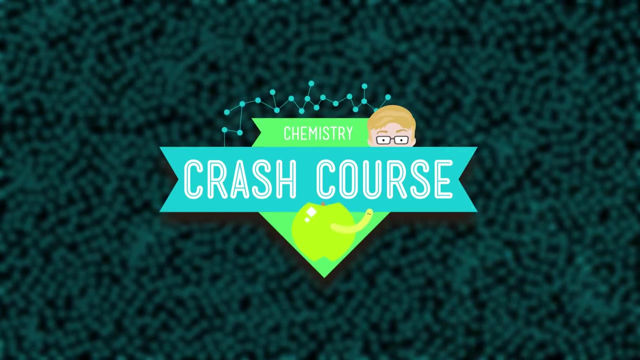 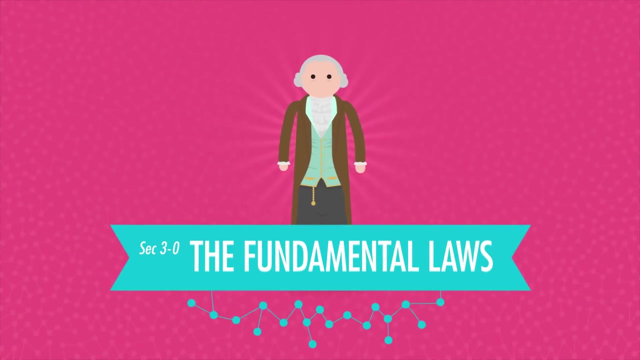 and you think to yourself: Gah, The guy who invented chemistry should be put to death. Well, you should feel bad, Because he was. Antoine Lavoisier was pretty fantastic. He was a geologist, a botanist, a biologist and a physicist. 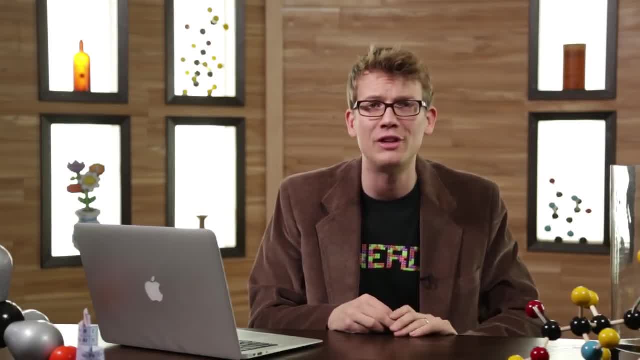 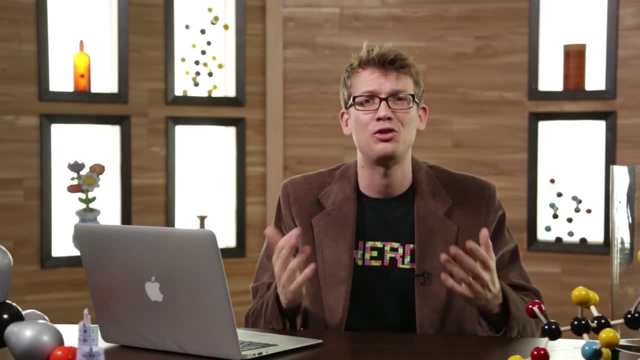 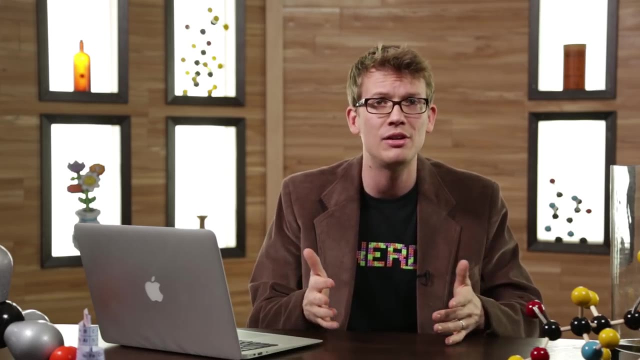 He helped define the metric system created in the international language of chemistry named hydrogen and oxygen. predicted the existence of silicon. outlined what elements were figured out, how animals extracted energy from food. determined that an element could take different forms upon discovering that both ash and diamond contained pure carbon. 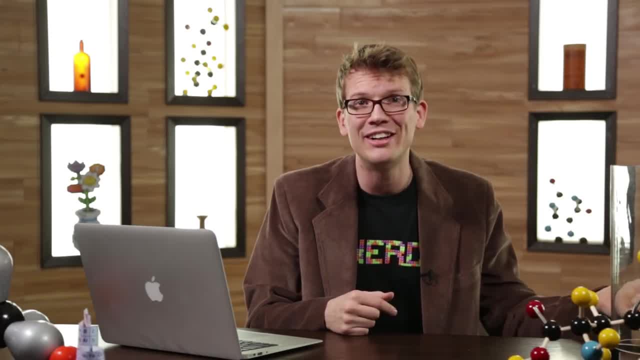 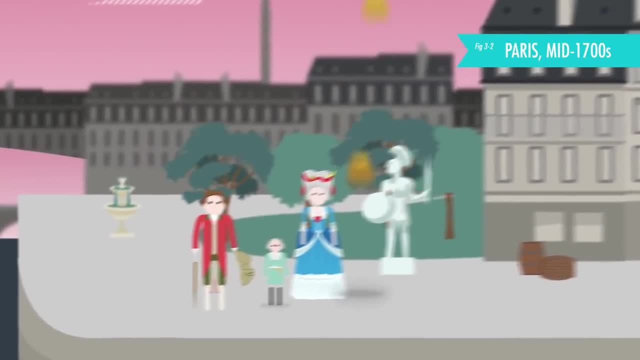 published the very first chemistry textbook ever, and there's a reason why the law of conservation of mass used to be called Lavoisier's Law. Born into a wealthy family, Lavoisier inherited a massive amount of money when his mom died, when he was five years old. 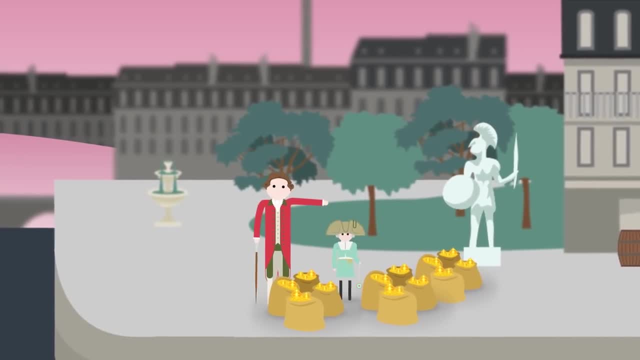 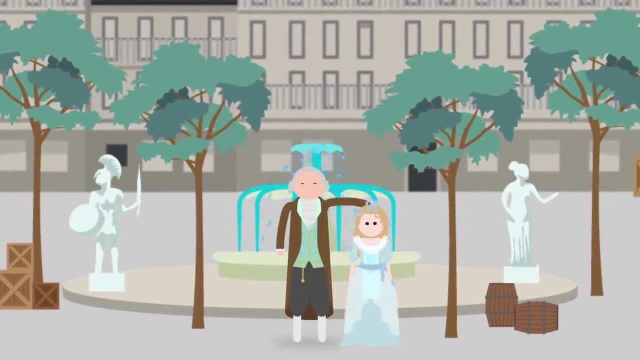 And though he did get licensed to practice law, as his father expected him to follow in his lawyerly footsteps, young Antoine chose science instead When the opportunity arose to marry a wealthy girl whose father's massive income came from collecting taxes for the French government. 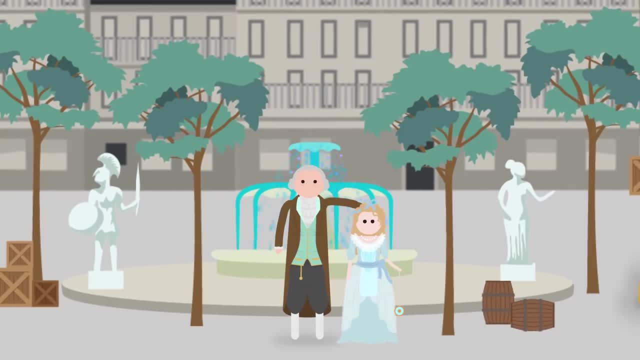 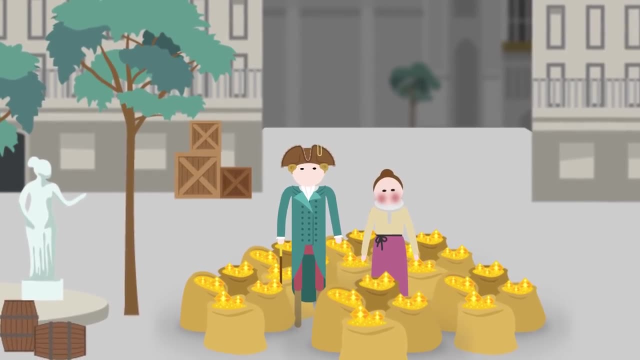 he did it even though she was 13.. A questionable decision, though not uncommon at the time. It turned out that the family connections would be his undoing, though not the age of the bride at her marriage. Marie-Anne, as she grew older, would become a colleague as well as a wife. 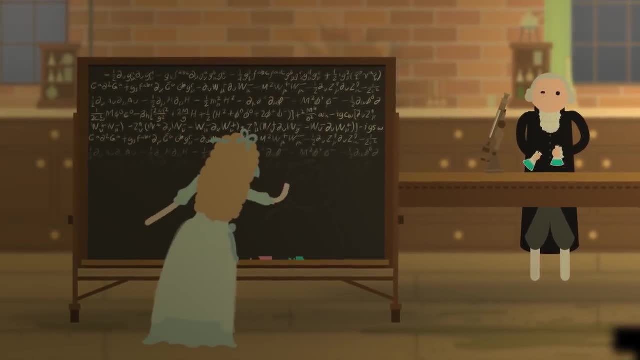 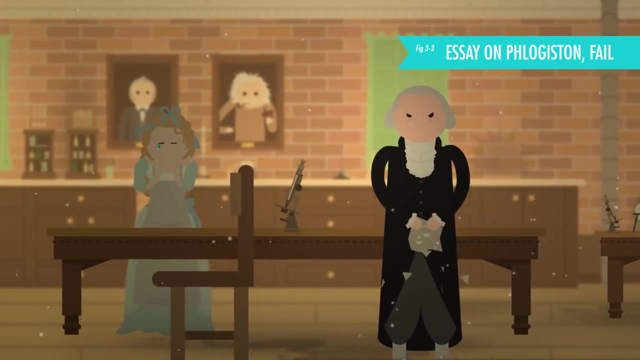 assisting Antoine in his experiments and his analysis of the work of others. Indeed, it was Marie-Anne who translated Essay on Phlogiston for Antoine, Which he ripped to pieces, changing everything forever, Until Antoine Lavoisier started inspecting everybody's work. 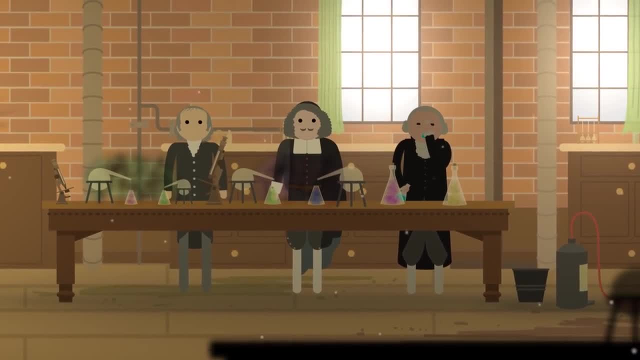 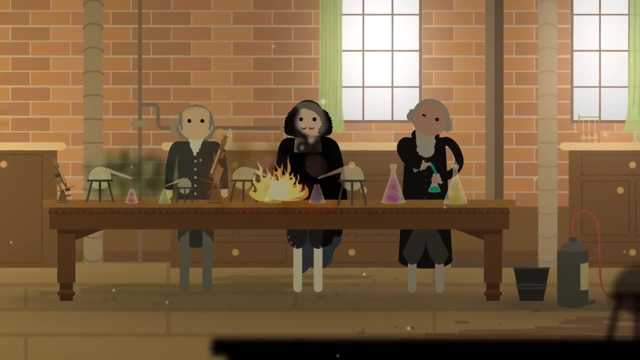 the prevailing theory of chemical change was that some substances contained an elusive element called phlogiston. By burning these phlogiston-containing elements, they would lose their phlogiston and become new things. Lavoisier took those theories and their research, combined it with research being done elsewhere. 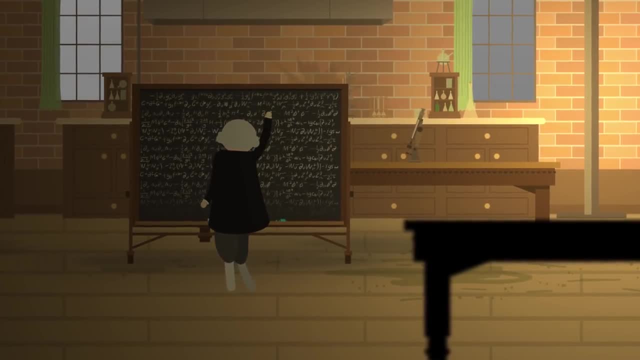 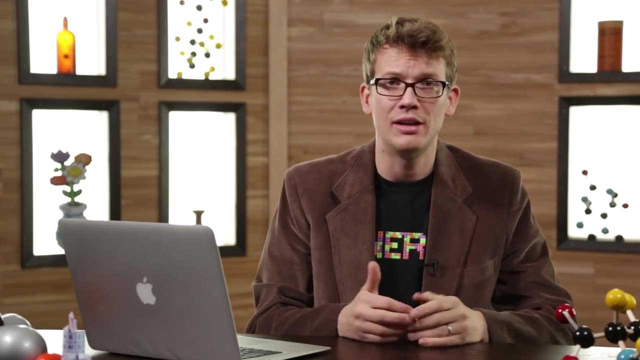 and added in his own genius experiments, and then tore the chemical world to pieces with a little thing called combustion. He determined that hydrogen wasn't inflammable air. it was an element. Indeed, he named it hydrogen because it was generated from water or hydro-generated. 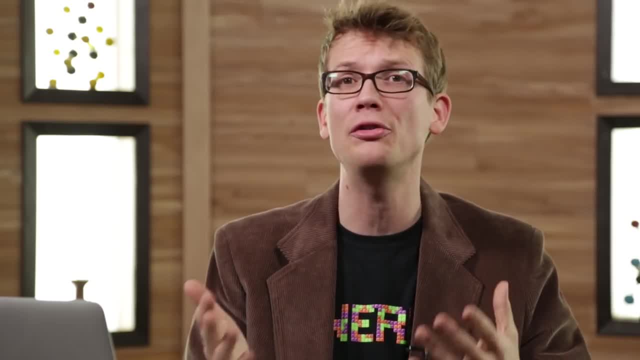 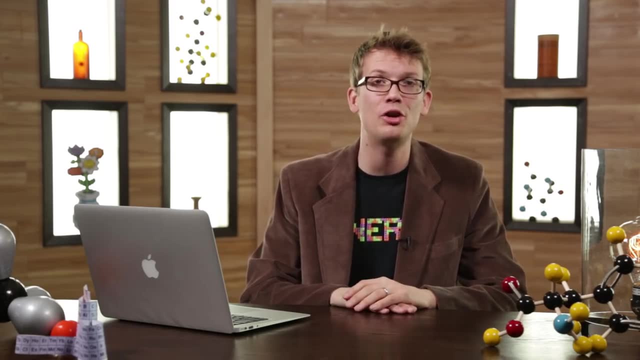 And he determined that oxygen was a vital ingredient for combustion and also what would later be known as oxidation, something that we'll discuss quite a lot in this course. By hooking people up to his bizarre contraptions, he determined that burning wood consumed the same amount of oxygen. 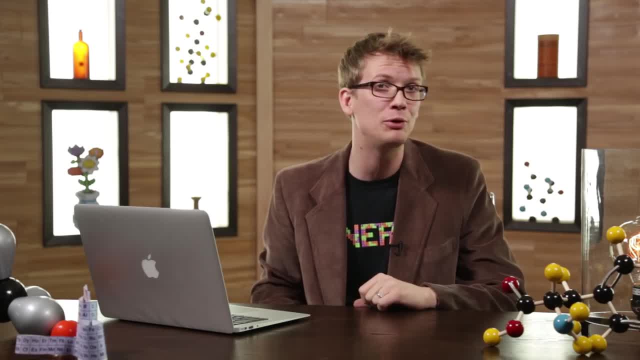 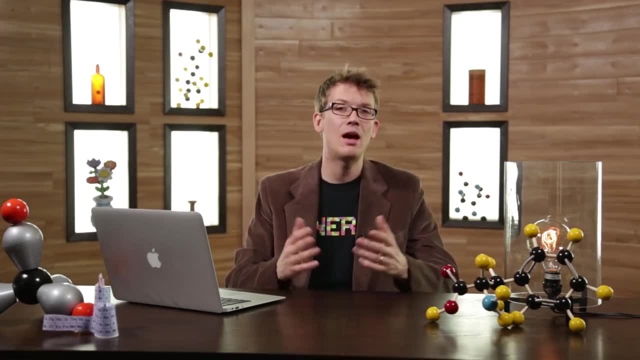 and produced the same amount of carbon dioxide as people consuming food and breathing, Thus determining that people and all animals are powered by some form of internal combustion. Now, experimenters of the day- I hesitate to call them chemists- notice that when you burn something, its mass decreased. 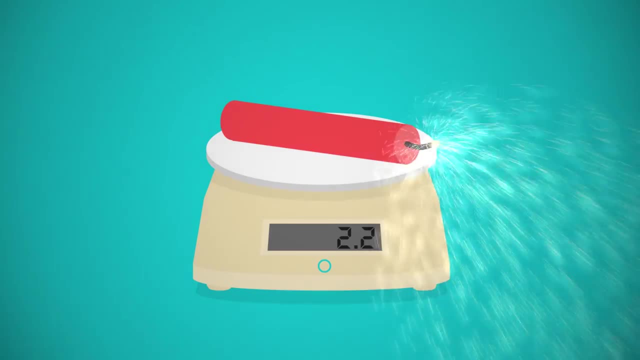 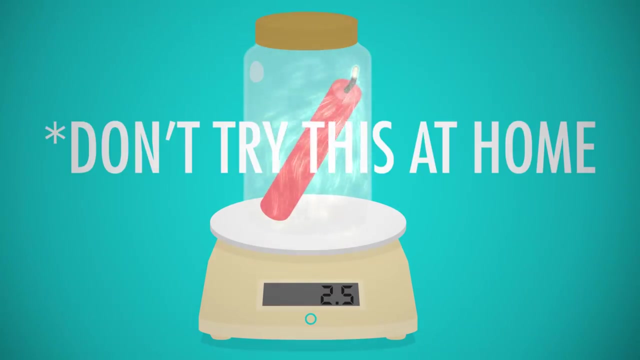 Like here's a fuse and I put it on a scale and I burn it and its mass decreases. But Lavoisier determined that if all the particles and gas are collected, like if I burn the fuse inside a closed bottle, the mass stays the same. 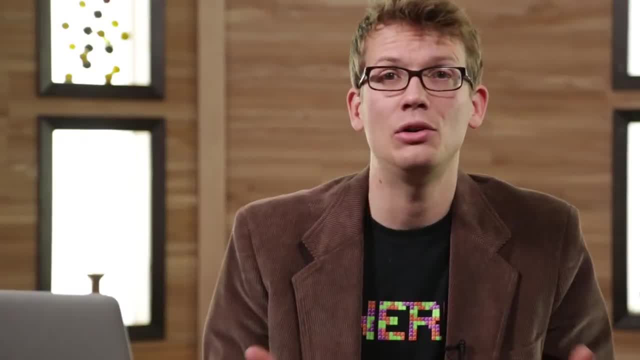 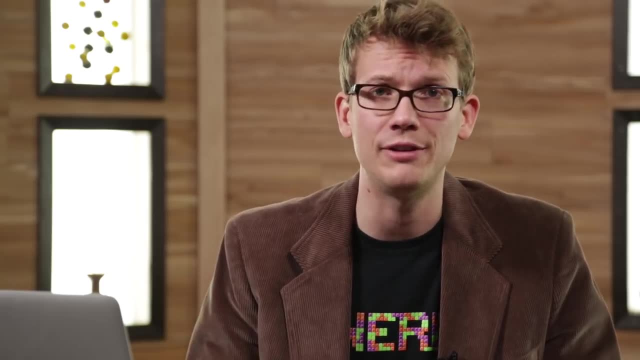 Stuff remained stuff. You can't lose any. You couldn't make more. This realization, though, it seems obvious to us now, and its acceptance by the general public and the general scientific community, as far as I'm concerned, was the precise moment at which alchemy ended and chemistry began. 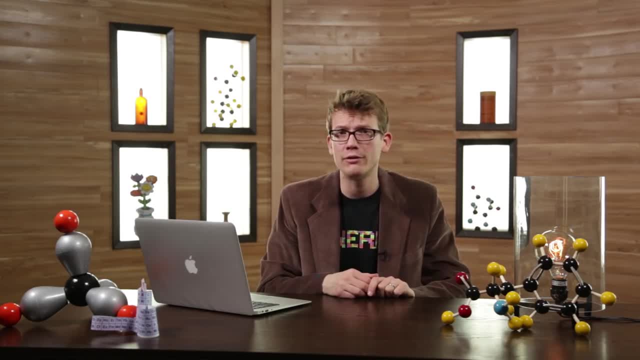 Lavoisier's chief contributions and ultimately his discovery of the law of conservation of mass, relied on careful measurement and careful thinking And, as you'll see, both of those things are key to success in chemistry. to this day, Lavoisier the man was a bit of a dichotomy. 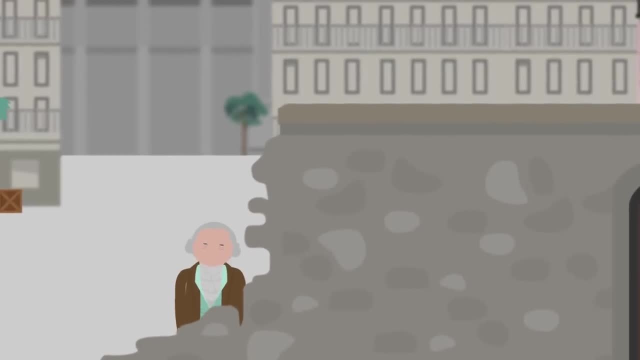 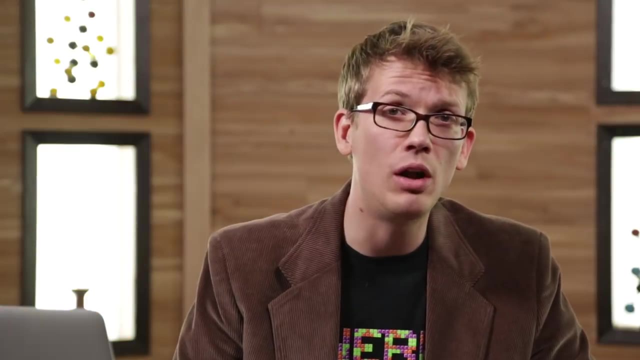 Having worked as a tax collector and helping to create a literal wall around Paris to assist in the collection of taxes, but also a supporter of the French Revolution as it began. But the enemies he had made with his wall and by denying certain powerful politicians entry into the French Academy of Sciences. 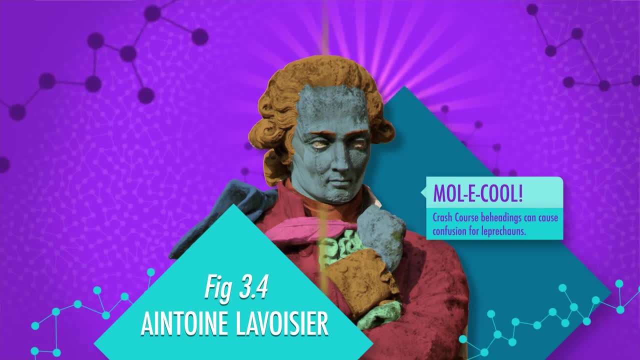 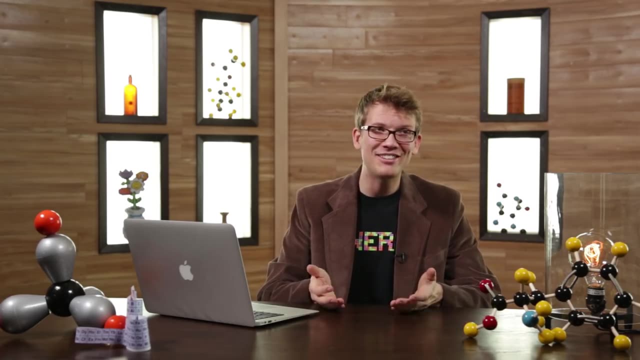 eventually caught up with him as the revolution's lunacy increased. He was beheaded on May 8th 1794.. Lavoisier was pardoned a year and a half after his execution. so that's good. Marianne was delivered all of his confiscated belongings. 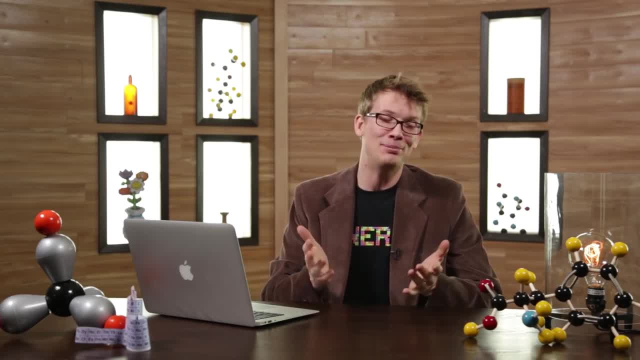 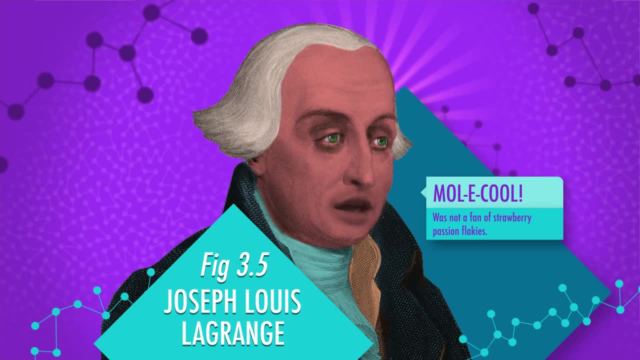 and a note of apology Like sorry we killed your husband. Here's all the stuff back. The mathematician Joseph Legrand said of the event: It took them only an instant to cut off that head, but France may not produce another like it in a century. 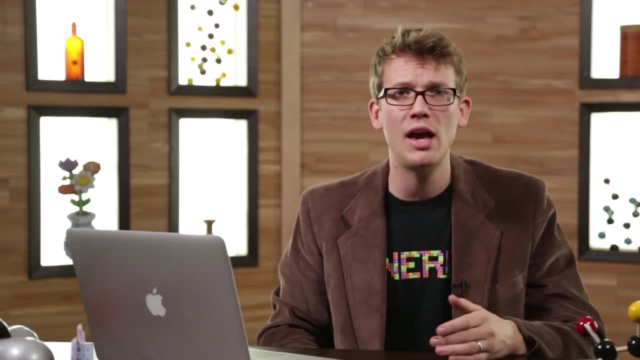 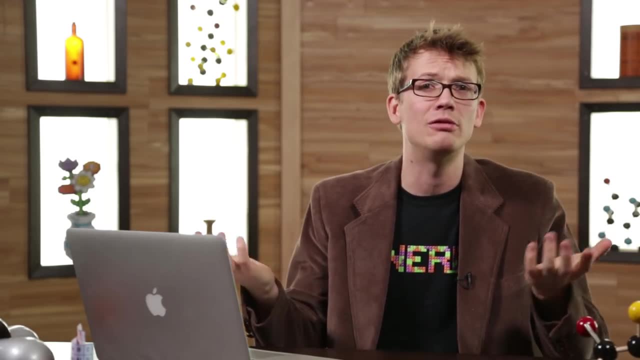 It's worth noting- though this isn't really science talk- that Lavoisier couldn't have done any of his magnificently careful measurements had it not been for his enormous wealth. He commissioned the creation of hundreds of pieces of equipment, large and small. 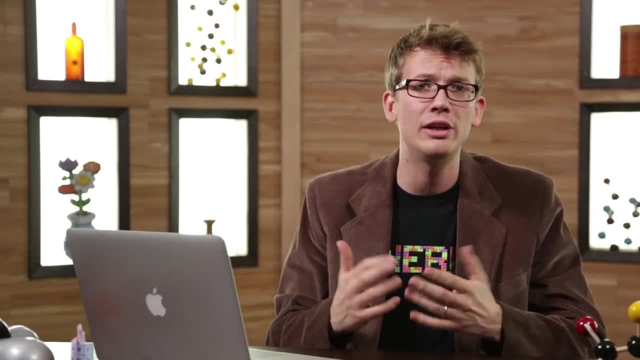 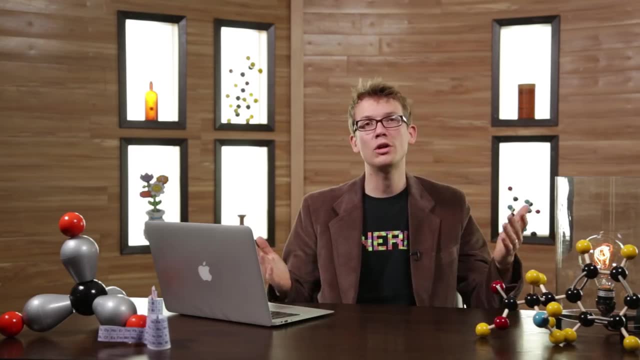 Only the system of economic inequality that the French were revolting against made it possible for Lavoisier to do his work. I'll leave you to think on the implications of that on your own. Lavoisier's work was, for a full century, the basis of all chemistry. 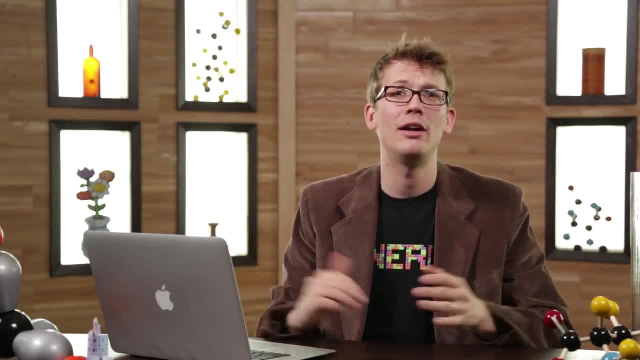 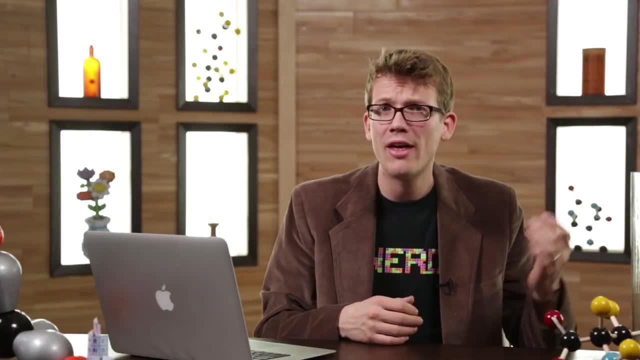 Proving that you don't have to be rich to get a law, at least temporarily, named after you. French pharmacist Joseph Proust built on Lavoisier's ideas of extremely careful measurement, showing that a chemical compound always contains the same proportions of elements. 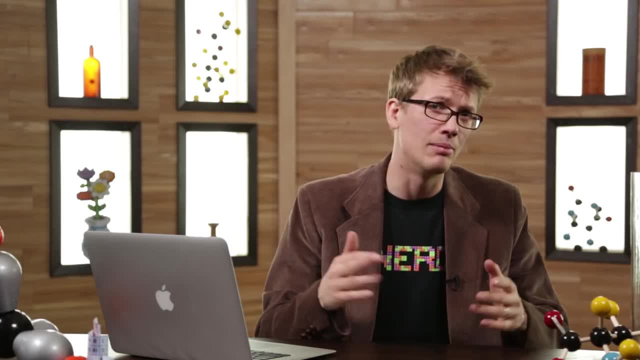 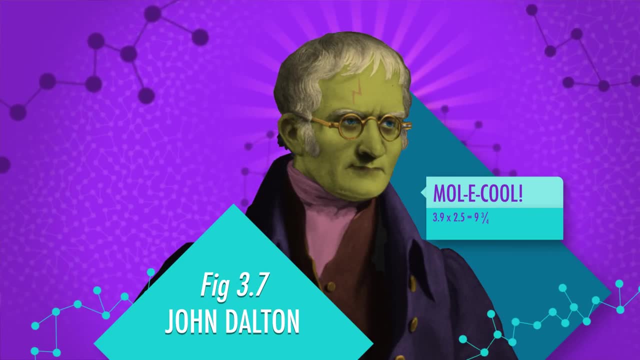 For a while we called this Proust's Law, but to make it easier to remember for the world, we just call it the Law of Definite Proportions. now And then an English school teacher, John Dalton, followed Proust by examining what at first, 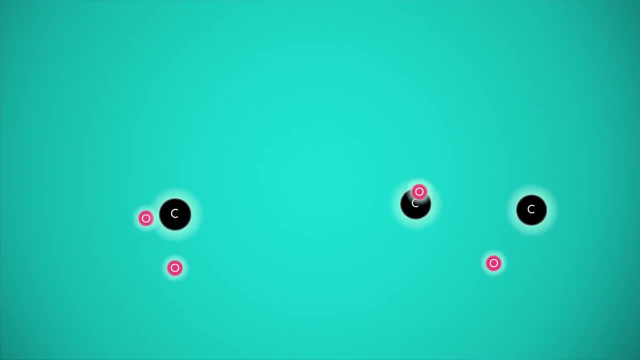 appeared to be a problem with Proust's work. Carbon and oxygen, when reacted together, would form two different proportions, not just one. Of course, what was happening is obvious to us: Carbon and oxygen were reacting to form two different compounds. 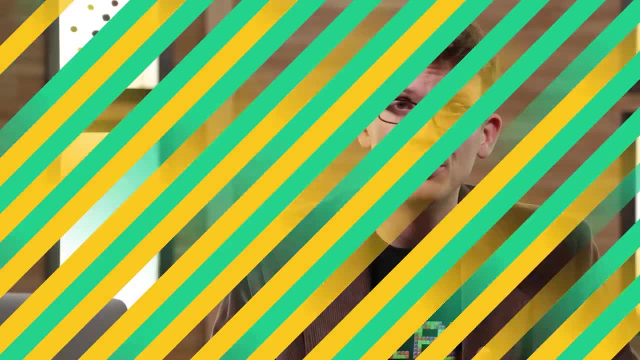 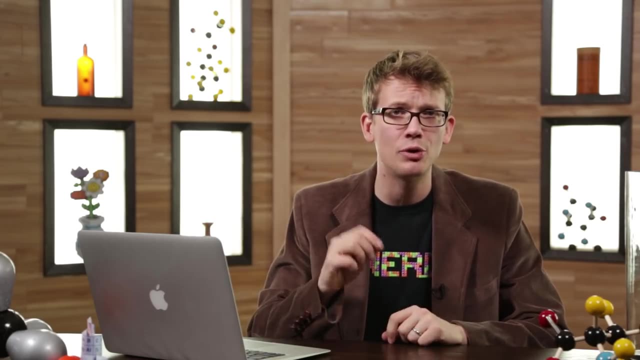 carbon dioxide and carbon monoxide. As Dalton's work continued, he found something truly mind-bendingly fascinating. If you limited the amount of carbon reacting to exactly one gram, the mass of oxygen consumed to produce one compound was 1.33 grams. 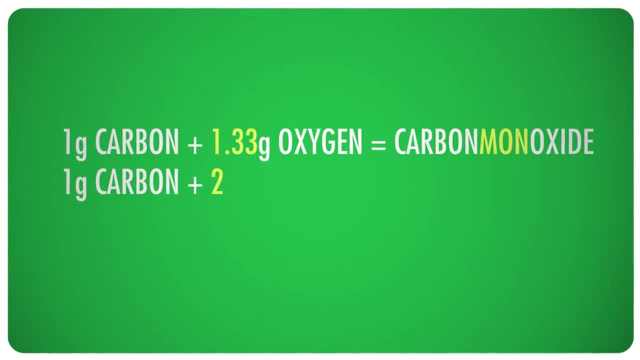 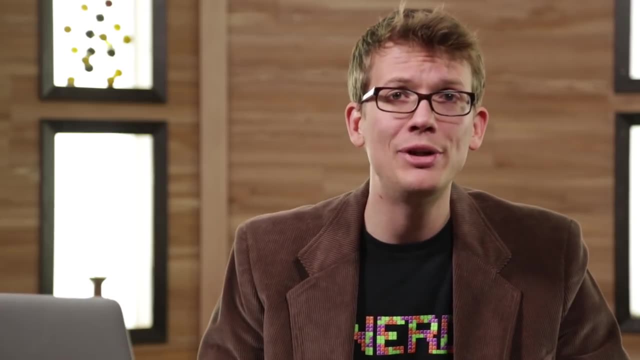 while the mass consumed to produce one compound was 2.66, exactly double what was required for the other compound. This shook out for other reactions too. When reacting nitrogen and oxygen, and limiting to exactly one gram of nitrogen, three compounds formed. 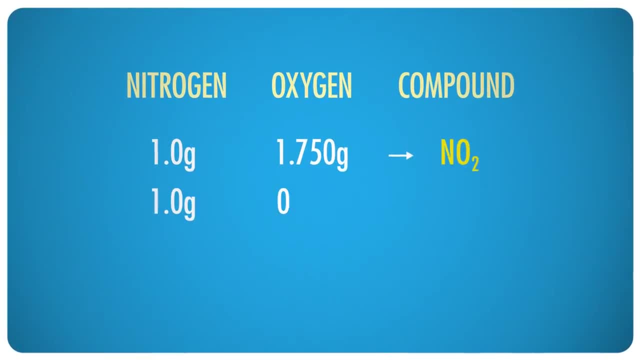 One compound consumed 1.750 grams of oxygen, another consumed 0.8750 grams and another consumed 0.4374 grams. All of those numbers are relatable by small whole-number ratios. Oxygen wasn't reacting with some ephemeral cloud. 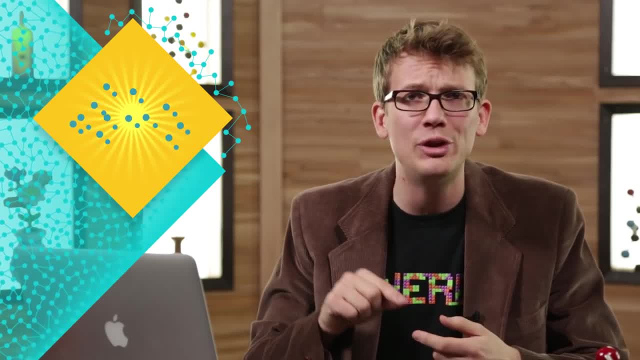 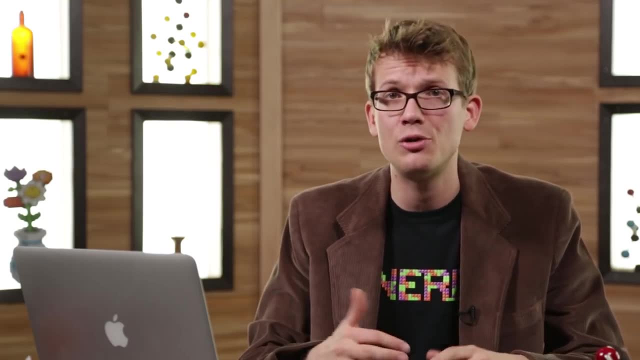 like the idea of nitrogen, It was reacting with individual, discrete bits of nitrogen that couldn't be divided. It could react in a number of ways, but it was always the same oxygen and the same nitrogen with the same properties. And so, while in our first episode we showed you how Einstein 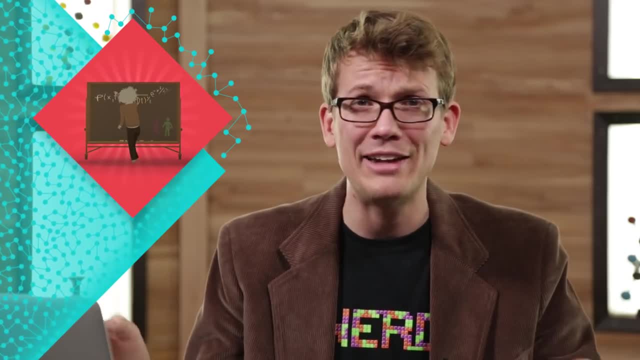 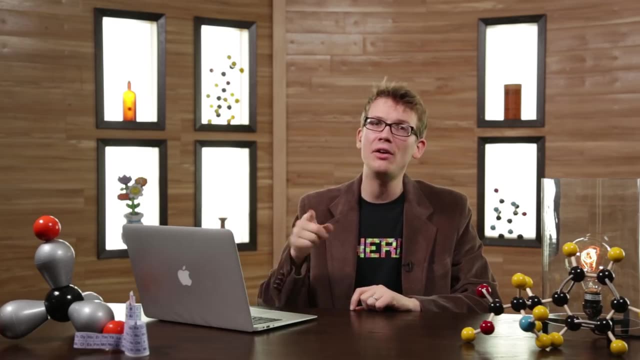 actually proved that atoms exist with super fancy math. Dalton had used multiplication to become the first person to actually have real data supporting the idea of atoms. Dalton still, though, had it kind of wrong. The products of his reactions were elements as well. 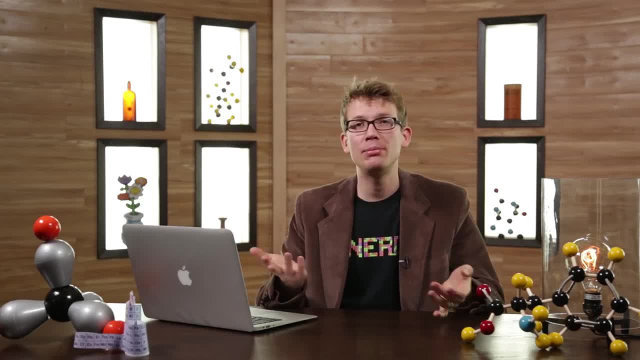 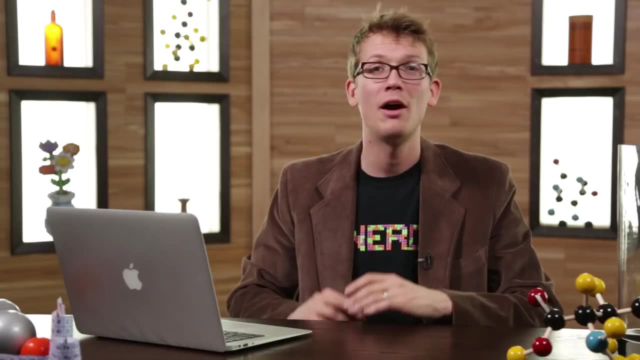 Basically, he believed that atoms and molecules were the same thing. We often simplify this and don't note Dalton's confusion on this particular point, but that leaves a couple of other fantastic chemists out of the story, For example Joseph-Louis Gay-Lussac. 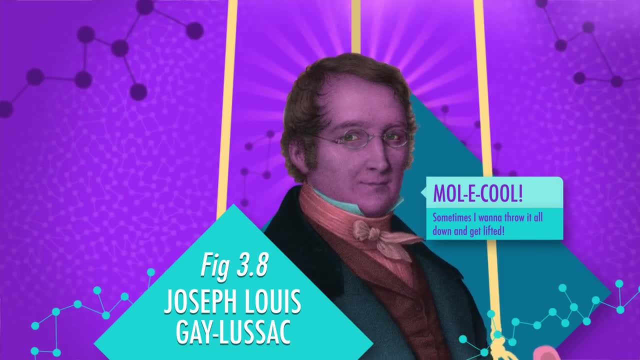 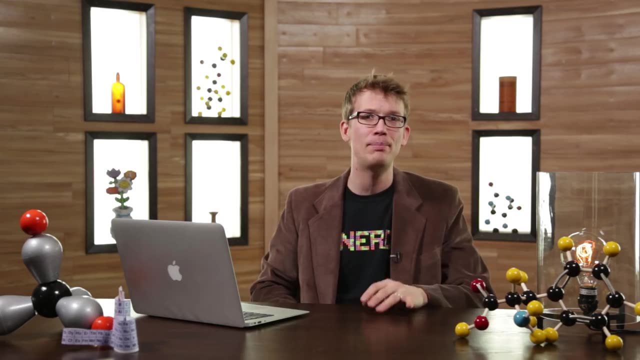 who, in 1804, became the highest scientist ever in history by taking a hot air balloon to the dangerous height of 7,000 meters to take air samples. But in addition to being maybe a little bit crazy, Gay-Lussac published a paper showing that a volume of oxygen gas 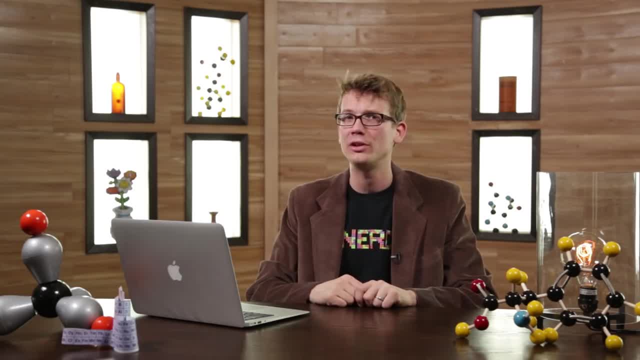 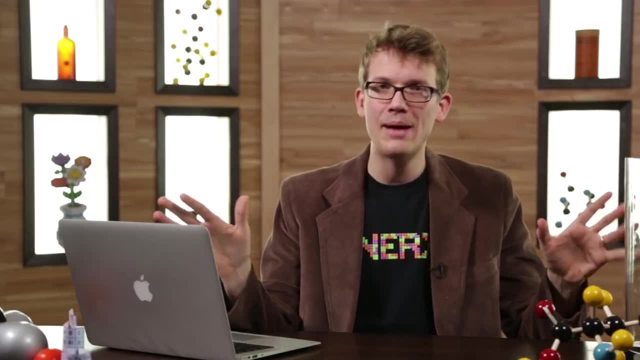 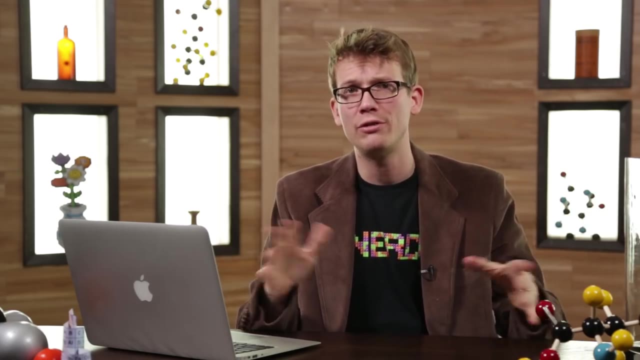 is two times smaller than the volume of water vapor it creates, indicating that somehow oxygen was splitting into two pieces. Dalton would not accept this, because it meant that oxygen was not one but two atoms, and apparently that just messed with his whole conception of the universe. 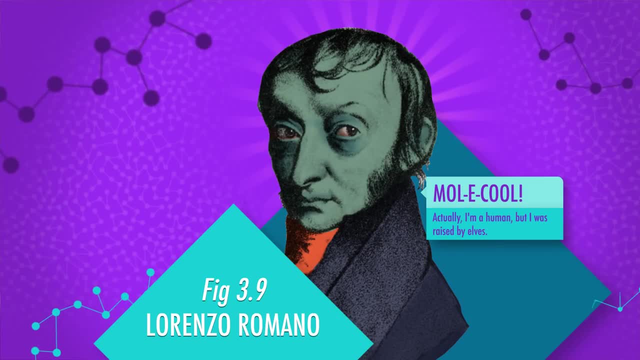 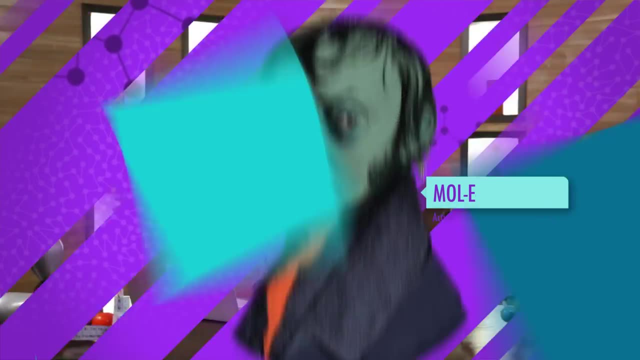 and he never did accept it, even unto his death. It took an Italian house-elf, I mean genius, Lorenzo, Romano Amadeo, Carlo Avogadro di Quaregna e di Ceretto. I did it the first time. 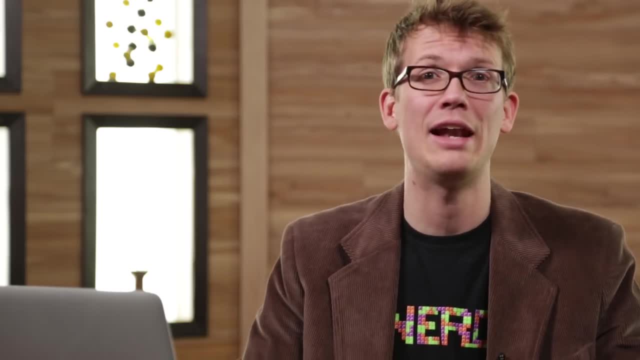 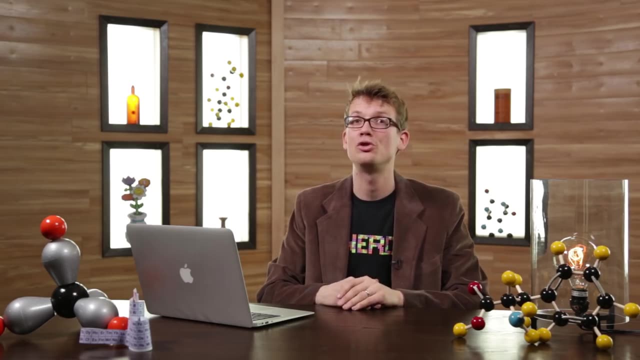 We'll just call him Amadeo Avogadro, but he was a count so he had to have a super fancy name- and I'm me, so I had to try to say it, Much like Lavoisier, Avogadro's political alliances would get him into trouble. 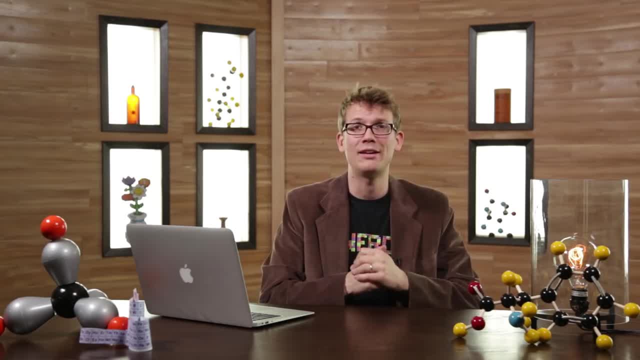 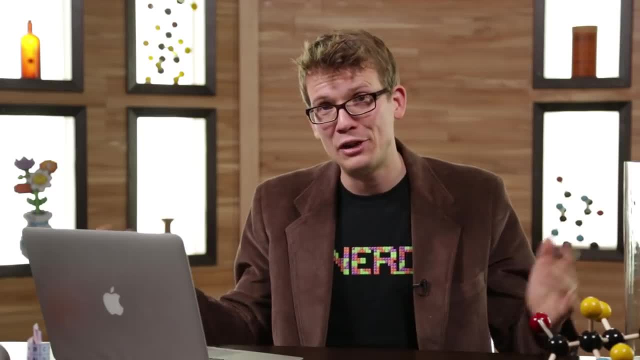 After Napoleon's downfall in 1815, Avogadro was active in the Italian anti-monarchy revolution, possibly even sponsoring some revolutionaries with his personal fortune. For this, he lost his chair at the University of Turin, but thankfully he did not lose his head. 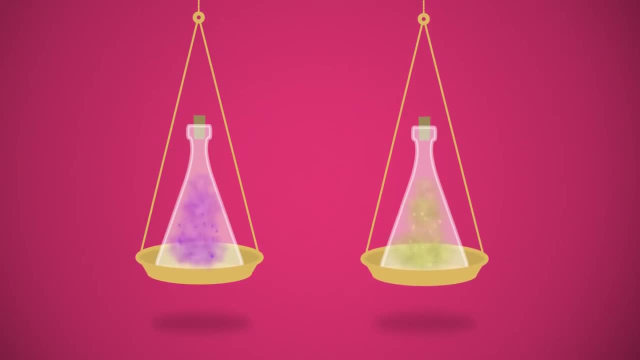 Avogadro proposed correctly that any gas in a container of the same size with the same temperature and pressure would have roughly the same number of molecules in it, no matter what the gas was. So any difference in mass between two flasks of the same size. 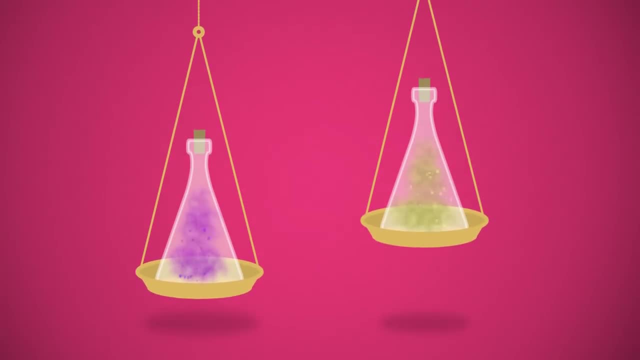 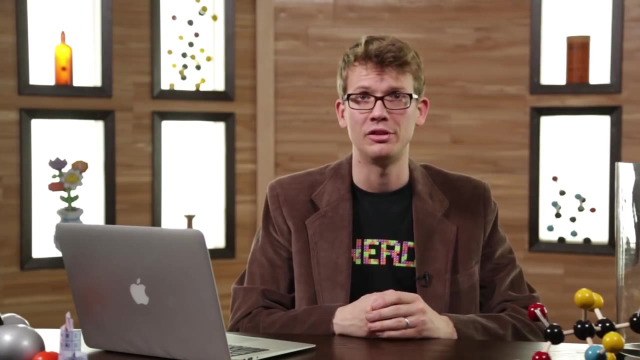 full of two different gases would be because of a difference in the actual physical mass of the molecules, And thus Avogadro basically figured out how to weigh atoms and molecules, as long as they were gaseous, To support his hypothesis, which was certainly good enough to support. 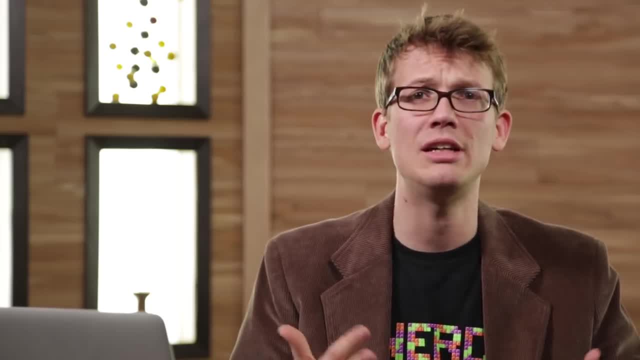 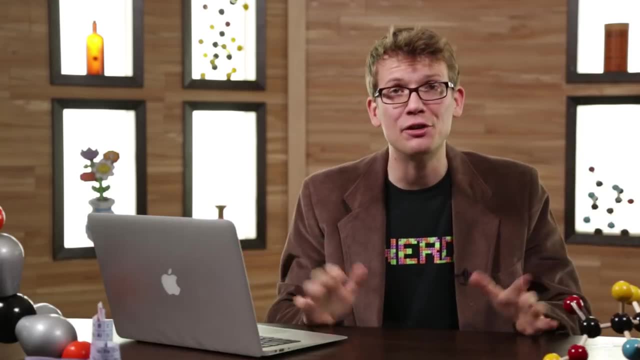 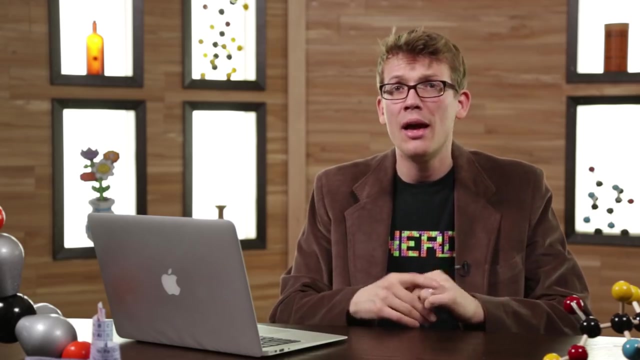 he suggested that in forming water, oxygen gas would actually split into two oxygen atoms, what he called elementary molecules that could not be broken down any further. For some 50 years Avogadro's idea of fundamental molecules were ignored, maybe because of incorrect ideas about how atoms stuck together. 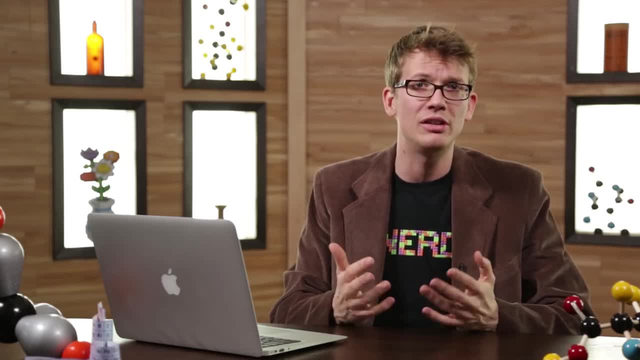 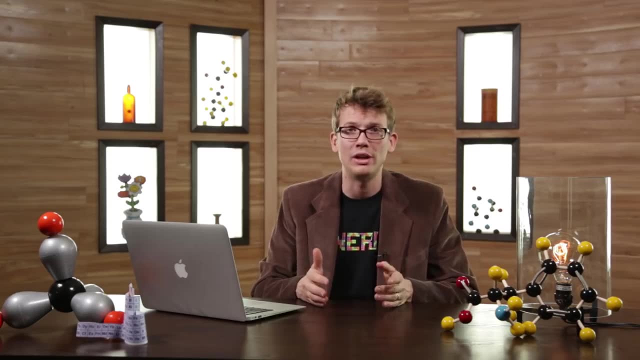 maybe because Italy was a bit of a backwater of science and Avogadro wasn't considered an important thinker at the time. But the scientific community, as it usually does, came back around to Avogadro's ideas eventually, not only naming his proposal that equal volumes at the same temperature and pressure. 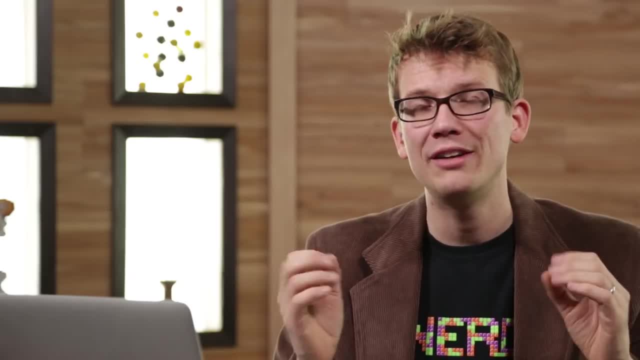 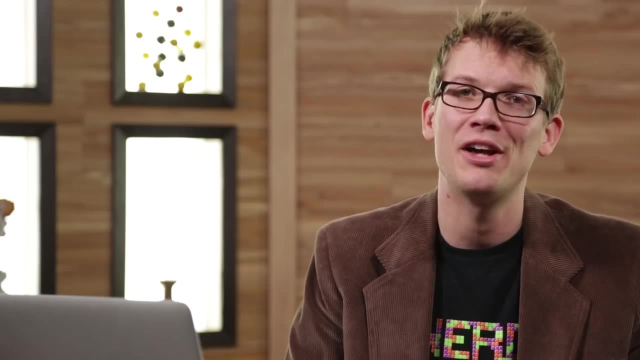 contain the same number of molecules. Avogadro's law, but also giving him his own number, maybe the most important number in chemistry, certainly one of my very favorite numbers, but we'll get to that later. Thank you for watching this episode of Crash Course Chemistry. 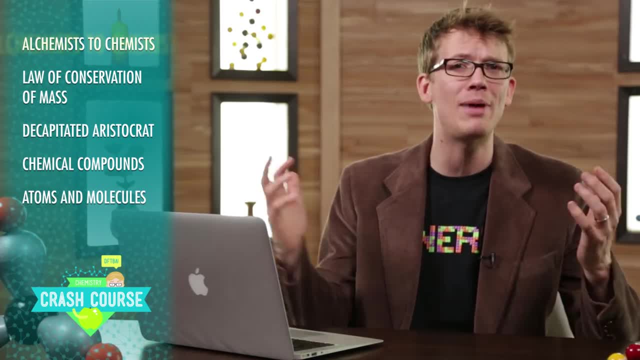 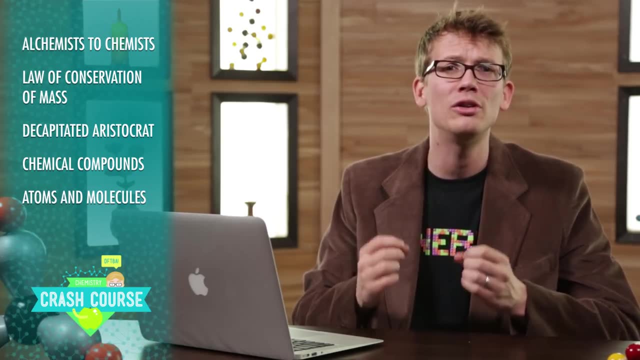 If you were paying attention, you now know the story of how we went from alchemists who thought that the element of fire hid inside of substances just clamoring to get out to chemists who understood the law of conservation, the law of conservation of mass, as proposed by a decapitated aristocrat. 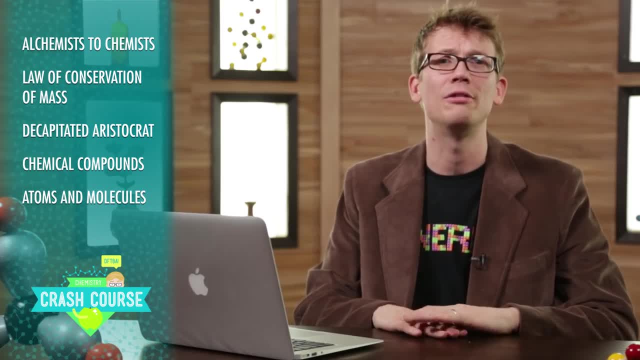 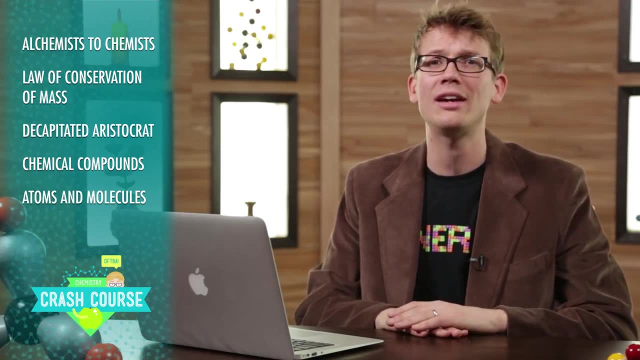 greater understanding of how chemical compounds work, thanks to a pharmacist and a schoolteacher. and eventually a complete understanding of what atoms and molecules are, thanks to a neglected Italian house self at Nobleman. This episode of Crash Course Chemistry: it was written by myself.